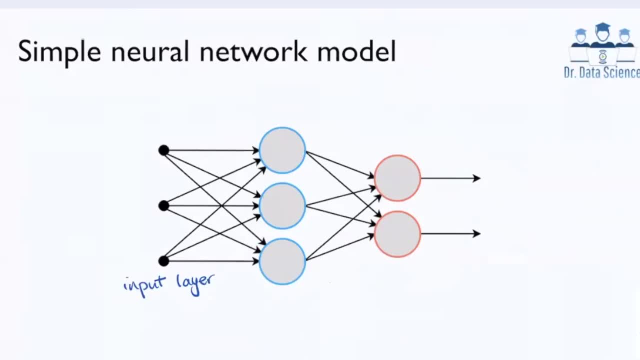 we have usually one or more hidden layers, So that's our hidden layer. That's where the magic happens, in the sense that we get the raw input data And we take this through some hidden layers before providing the output values. And here, in this simple case, I have only one hidden layer. 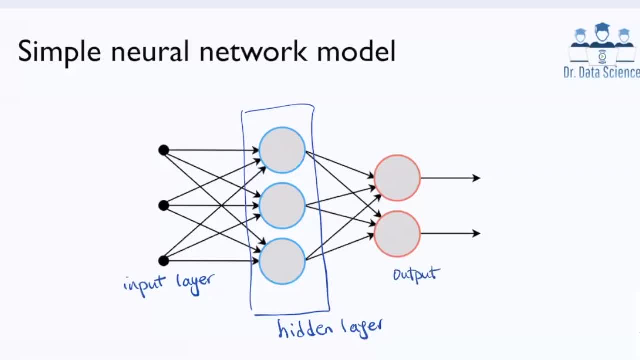 And this is the output layer. So in some cases you might have more than one output variable. Let's say you want to both figure out if there is a cat in an image and also you want to see if there is a dog. So each of these they need to have one output variable in the last. 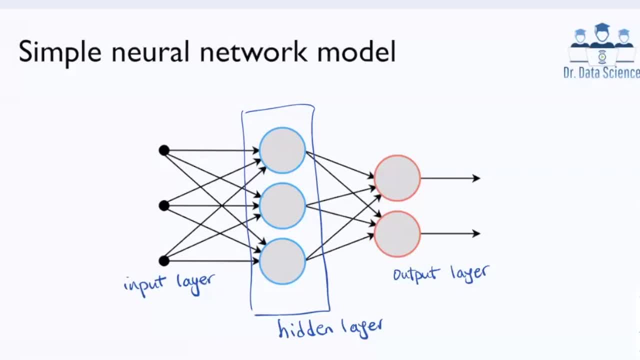 layer. So that's the general format, And when we have the weights for these connections, for these connections that you see here, it's very easy to find the output right. You take the inputs and you have this propagation through the network until you get the output. 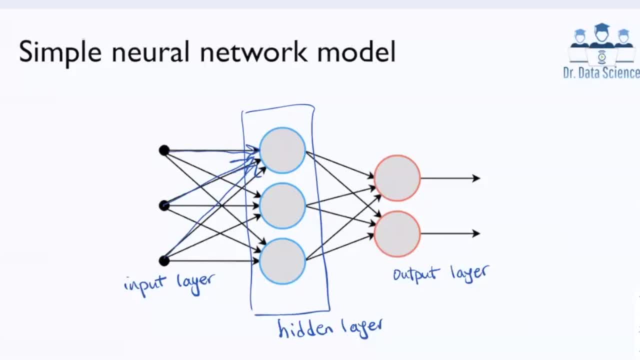 But the key idea is that we have to be able to find appropriate values for these weights, and that's when we have to use optimization techniques And that's where backpropagation becomes important. So for now, let's say we want to solve this problem And, because this might, 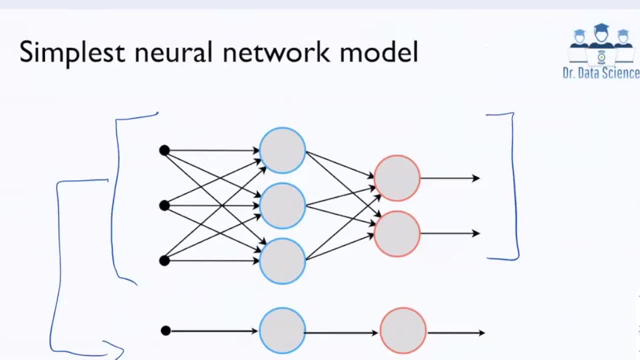 look a little bit complicated. I just simplified this to convey you the main message behind backpropagation. So what I did here to simplify this, I assumed that in each layer I only have one neuron, right? So I have one neuron in the hidden layer, the blue one, and one neuron in the 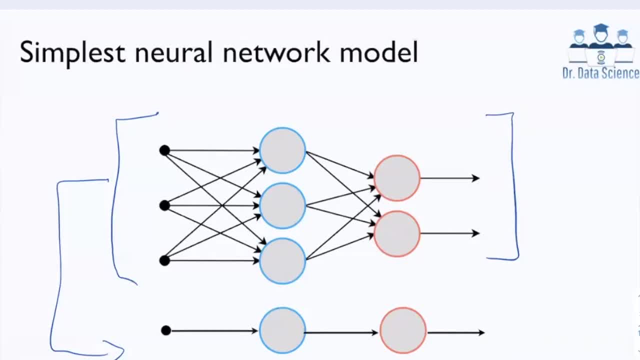 output layer, And also here we have the only like one input variable. You can extend this idea when you have more than one neuron, but then that's the point, that you have to use a lot of indexing and things get complicated. So if you're trying to understand backpropagation, in my opinion the 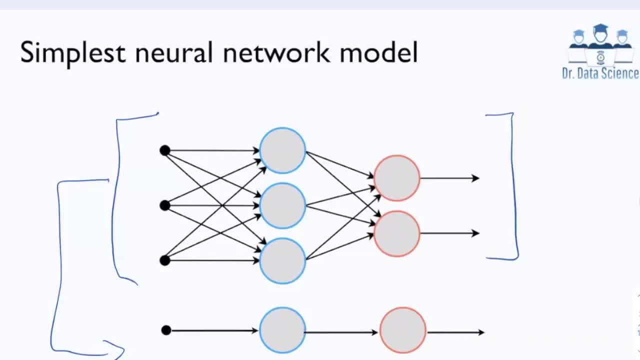 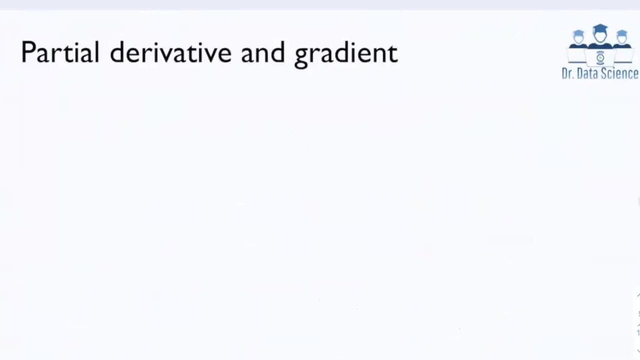 best way is to consider the case that you have one neuron per layer. But even before we are going to use this simply a simplified model, I want to tell you a little bit about partial derivatives and gradients, because that's something that we need and something that you may not already know. So why? 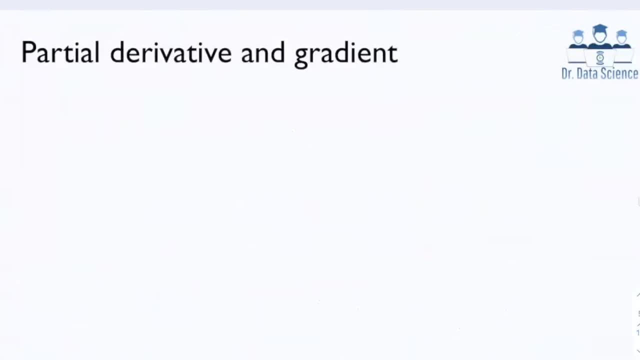 we need to use partial derivative. So, as we said, you only have a function f of x equals x squared. You know that the derivative of this function with respect to x is equal to 2 times x. And remember, derivative is something that tells us about the rate of change, right? So it means that if x, 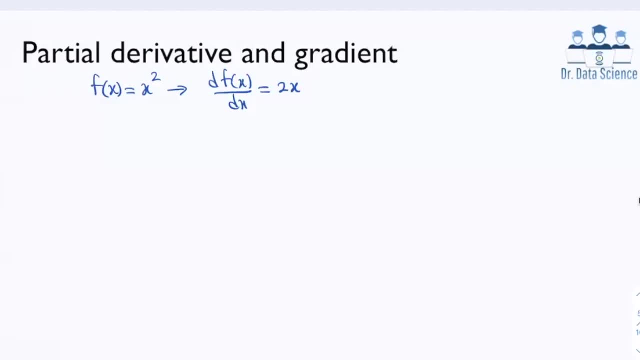 changes how this function f of x will change. However, in many cases we might have a function that has more than one variable right. So here we have x1 and x2.. So let's say this function is x1 squared plus x2 squared right. So obviously this is a variable right. So we have a function. 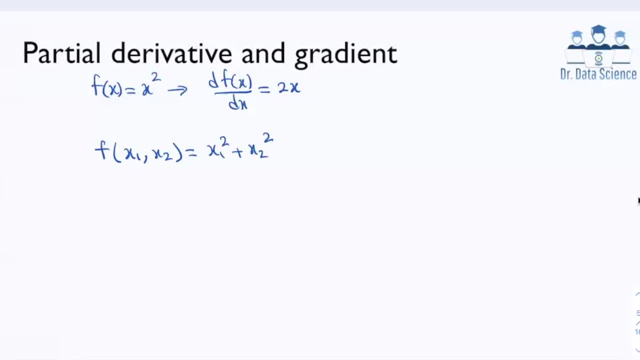 that has a valid function. We have two variables, x1 and x2, and this is the form that we have. So now, if I want to find the rate of change, you may say that whether I have to change x1 and x2,. 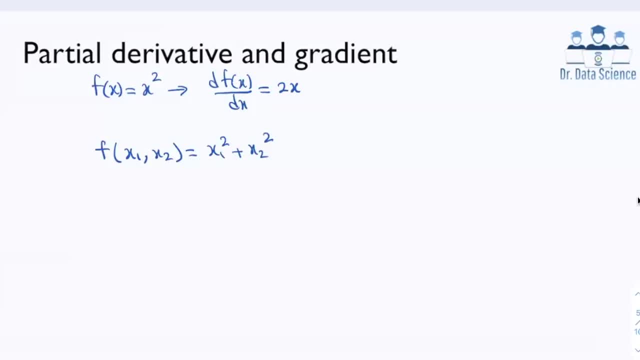 and that's where we have to use partial derivative. So let's say, I want to find the partial derivative with respect to x1.. And, by the way, this is a notation that we use for partial derivative, So we are not going to use d as we did before. We use this. 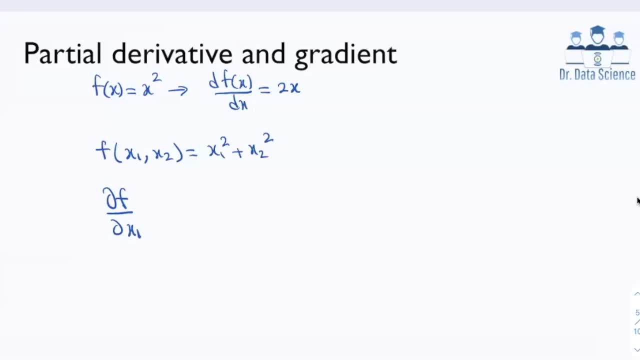 partial notation. So that's the notation we use for partial derivative. So what this means is that when we want to find the partial derivative with respect to x1, we assume- that's the key word here- that x2 is constant. So that's the assumption that we make. So if x2 is constant, let's say: 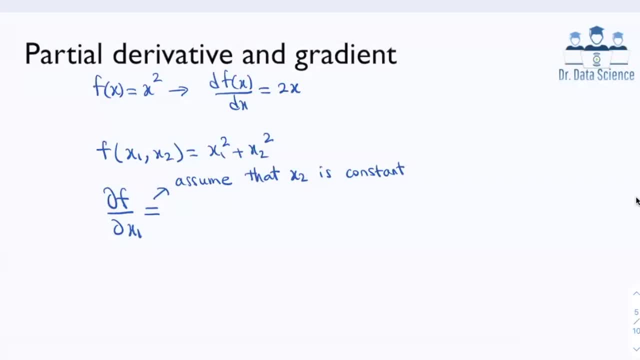 it's one or two, any number that you want to pick, any constant value, then what happens is that I get here x1 squared, and I know that the derivative of x1 squared with respect to x1 is two times x1. And then I have the partial derivative of x2 squared with respect to x1,. 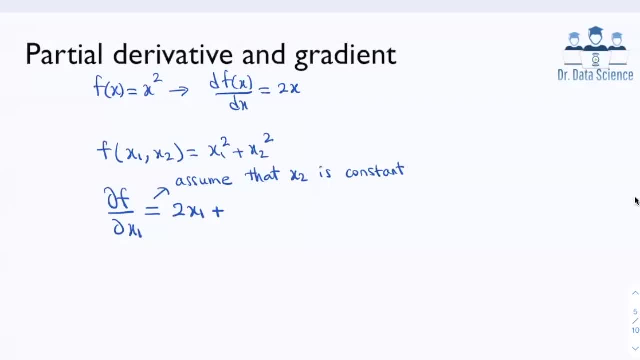 but remember: x2 is constant. And what's the derivative of constant? It's zero, because constant doesn't change. So that means that the partial derivative is equal to two times x1.. Now I can do a similar thing for partial derivative with respect to: 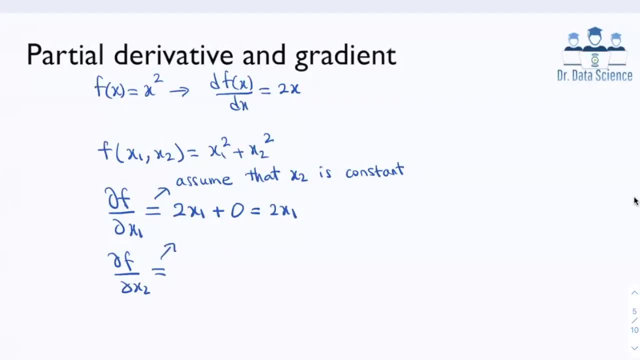 x2.. And, similar to before, I assume that the other variable, which here is x1, is constant. So now I have to find the partial derivative of x1 squared with respect to x2, and x1 is constant, So it doesn't change. So that's zero Plus partial derivative of x2 squared with respect to x2,. 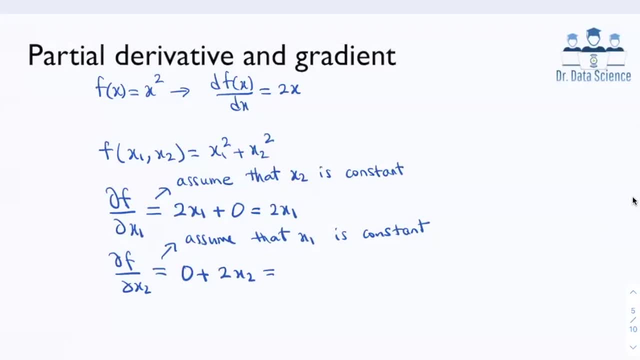 which gives me two times x2.. So in general you may have a function with more than two variables. You might have like 10 or hundreds of variables, And the key thing here is that now I can define something called the gradient. So that's the gradient. 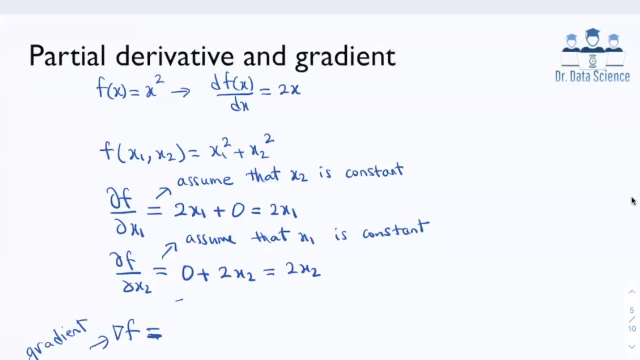 Which is an array that includes all these partial derivatives. So it means that here the gradient has two elements, because I have two partial derivatives, And the first element is 2x1, as we calculated, and the second one is 2x2.. I can factor these two, So I get 2x1x2.. 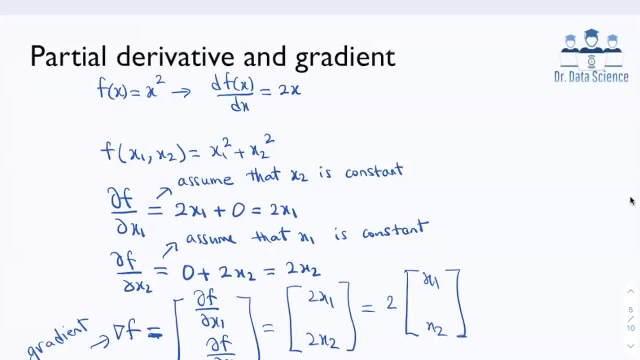 And what this basically means is that if I have this function f, which has two variables, and I want to find the rate of change, I have to find the rate of change with respect to each variable separately. And these are the values. So, with respect to x1, is 2 times x1, and with respect to x2, is 2 times x2.. 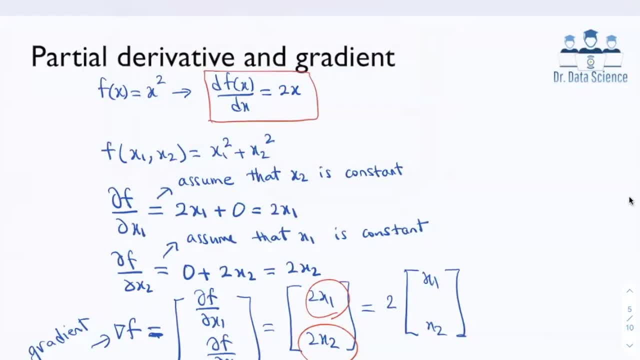 Right, And that's something that we can see from here too. right, Because we know that if I have just any type of like quadratic form, x squared, the rate of change is 2 times x, And so now I have this f of x1 and x2, which has this form of x1 squared plus x2 squared. 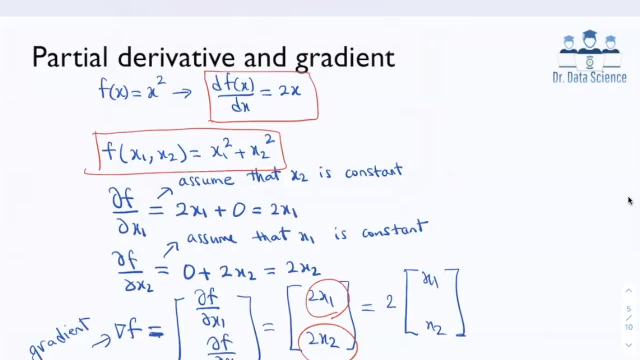 So this means that with respect to x1, rate of change is 2 times x1, and with respect to x2 is 2 times x2.. So now you may want to wonder why even we care about gradient. The reason is that. 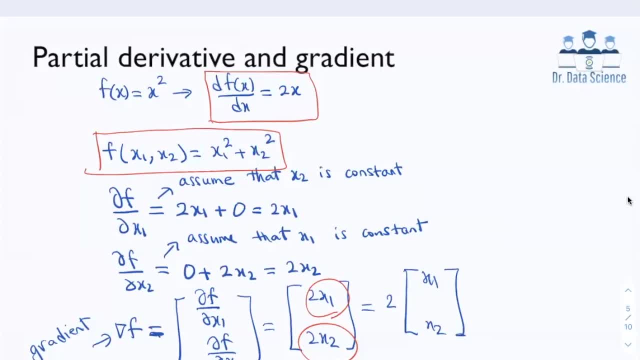 in order to find the weights of those connections in neural networks, we have to use optimization methods. So we have to find the weights of those connections in neural networks, We have to use optimization methods, And the most commonly used optimization method is gradient descent and its variance. 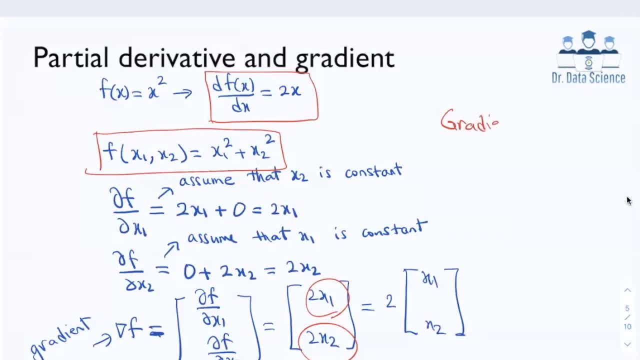 So what does gradient descent does? is that we are going to have some estimates. So in general, let's say, I have some estimate of the solution and then I'm going to move opposite direction of the gradient and that's what gives me the new update. So this is your. 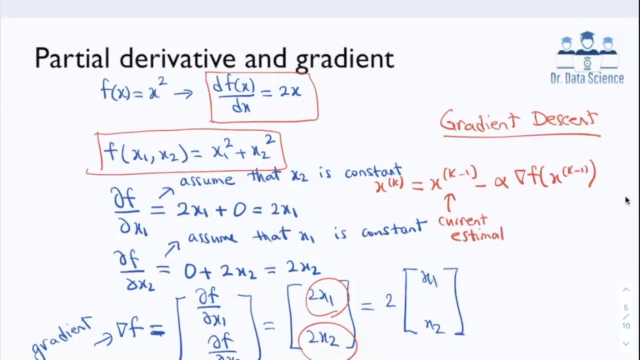 current estimate. This is the gradient, And alpha is just a positive constant. And the intuition is that, let's say, if I have a function that looks like this, I obviously here use only one variable to just make it simpler to visualize this. But if I am here and I want to figure out whether I should go to right, 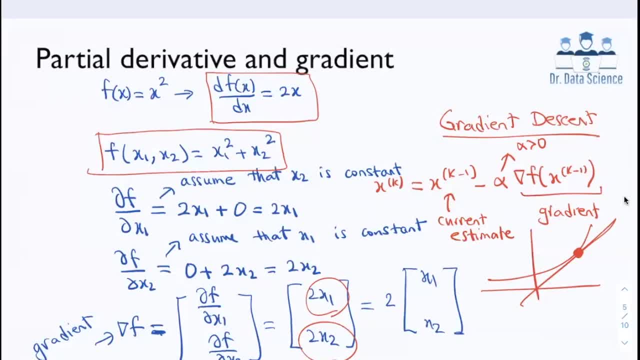 or left to decrease the value of this function. I have to go to the opposite side of the derivative or gradient when you have more than one variable. So this means that I have to go to this side. So that's why I have, like this negative sign here. 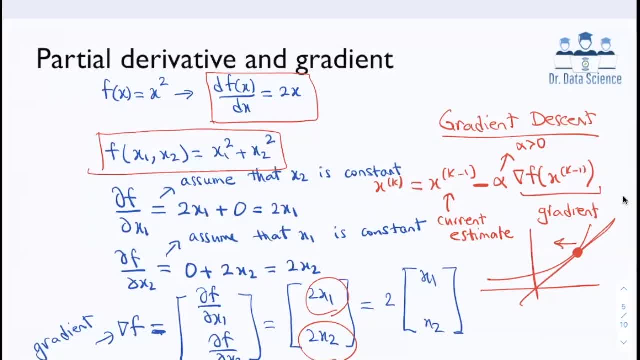 And that's the general idea behind gradient descent that we use for optimizing the weights of neural network, And that's the general idea behind gradient descent that we use for optimizing the weights of neural networks. So I'm going to make another video to discuss more about this gradient descent part. I know that here. 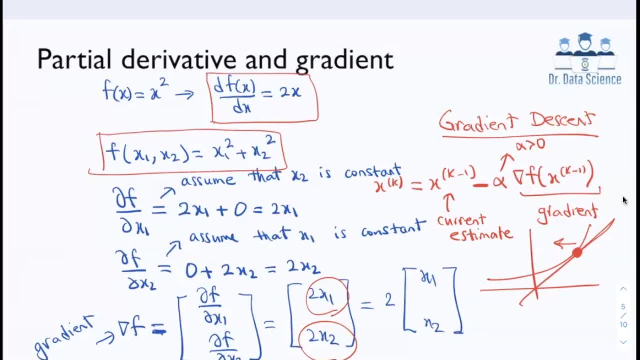 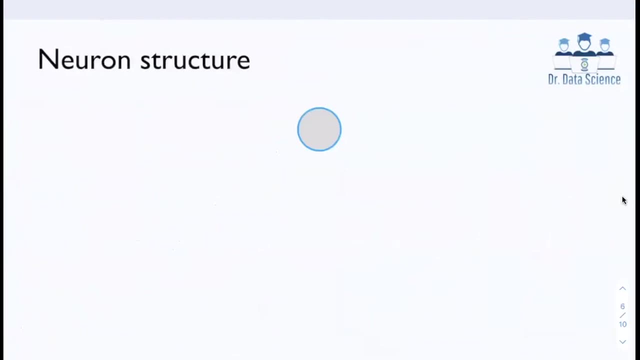 I just talked about that very briefly, but my idea here is that, to show you that, why we care about the gradient and partial derivatives. Okay, so, with this in motivation in mind, we have one more step to go back to that simplified neural network model that we have. So, if you remember that, 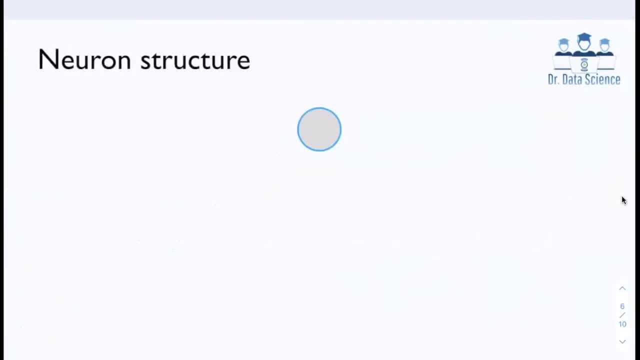 neural network had a lot of neurons in it, right, So it is important to understand how these neurons work. So the way that they work is that it's a little bit confusing because we are not showing the full picture. So the way that this works is that this has neuron, has two parts, A summation. 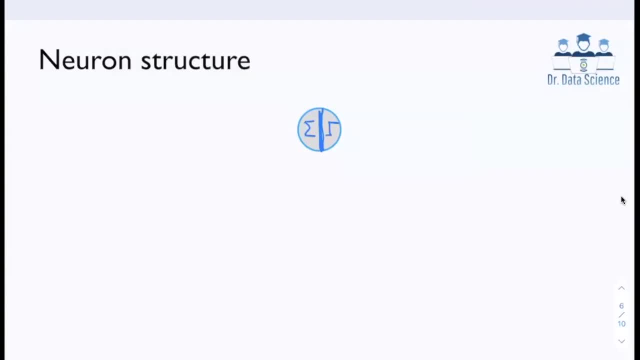 part and then what we call as activation function. So let's say we have three inputs to this neuron, and here I just call them x1, x2.. x3. Usually neurons in the middle layers or intermediate layers they don't get inputs from. 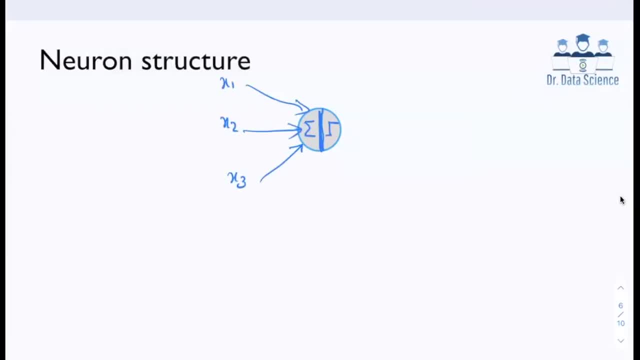 the from the raw data, but they get from the previous layers. But for now let's just assume that these are the inputs and let's say these are the weights: w1, w2, w3.. So this first part which is here computes something that we call it z here, which is w1 times x1, w2 times x2,. 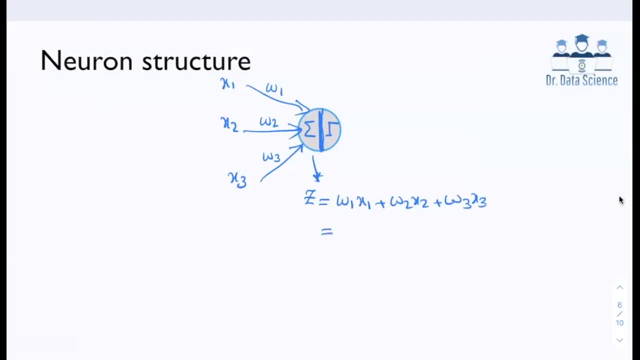 and w3 times x3.. We can also use a summation notation, so that we can see why I use that notation there. So that's wi xi i equals one, two, three. If you feel more comfortable with linear algebra, you can also create two vectors, w and x, and then find the inner product between. 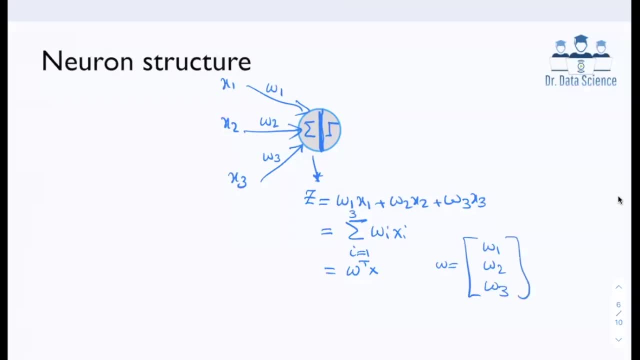 these two vectors. So that's how this last line looks like. So we have two vectors and now we find the inner product between these two And then the other part of this neuron. the second part is that we're going to apply these. 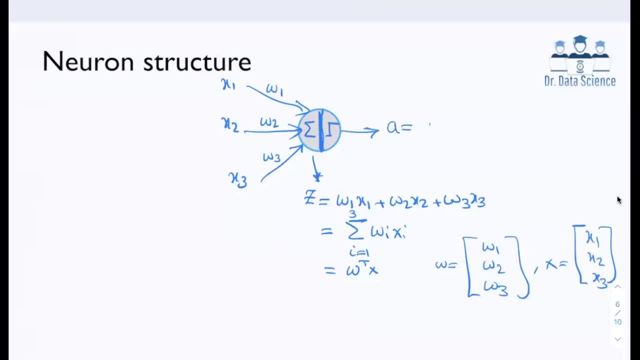 activation functions. That's the way we show it using a, and now we have this function, which I show here, with phi and then phi of z. So that's something important to remember here. So z is what we have here and a is what this neuron produces, which is simply phi of z. I could 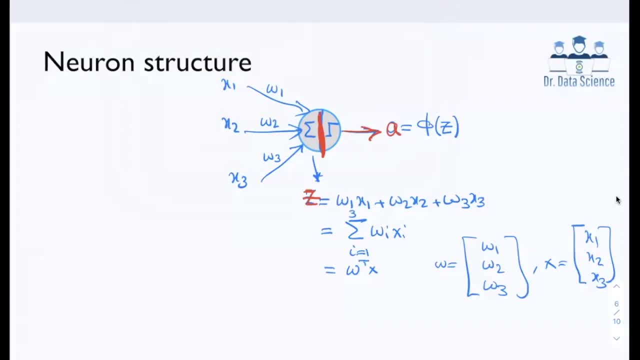 obviously put this together and say that a is equals phi of w1- x1 plus w2- x2 plus w3- x3.. But I don't want to do that because that will simplify things in the next slide when I'm talking about back propagation. 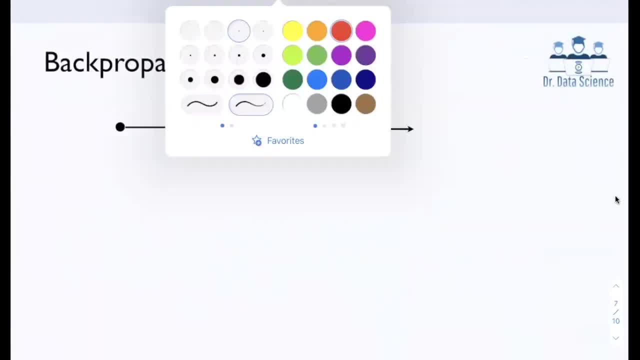 So, having this in mind, let's go now to the model that we had before That, as we said, we have one neuron per layer. So, in order to name this, I call this x, right, I call this w1.. So w1 is the weight that goes from. 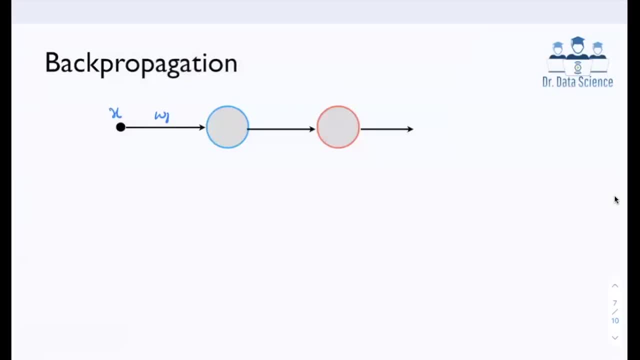 the input layer to the hidden layer, And then I call this weight w2, right, So this is w1, this is w2 and the output of this neuron is A2, because here let me use a different color. I use like a red color here to show that. 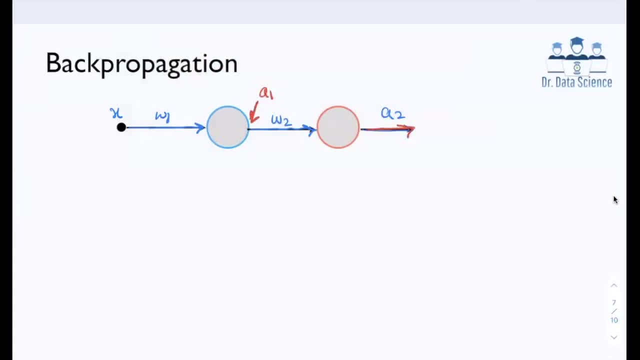 So here we have A1 and here we have A2. And I don't really show here Z, because Z is basically inside these neurons that we had in the previous slide. One way I can do this actually to make this simpler- is to again show what we had in the previous slide. 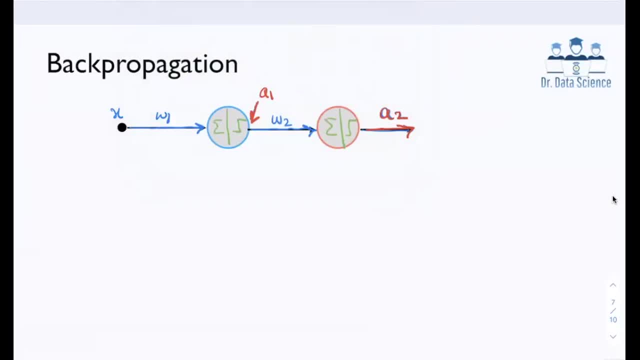 the sigma notation and the function that we have. So here we can see that we have- I show it here- Z1, which is W1X, and Z2, which is W2 times A1.. And that's the point that I made in the previous slide. 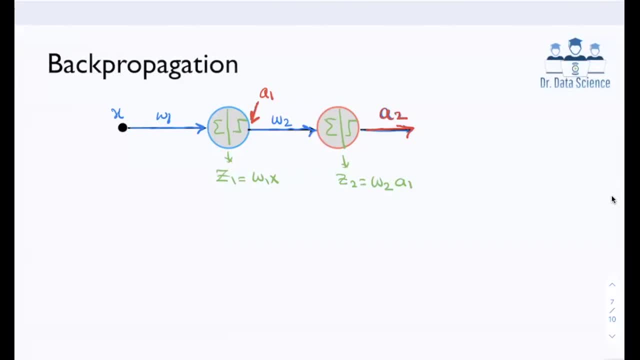 that for this red neuron, if you look at it, this gave the input to this is from the previous neuron which outputs A1. So we multiply A1 by W2, that's what we give us Z2.. And then we know that A2 is equals to phi of Z2.. 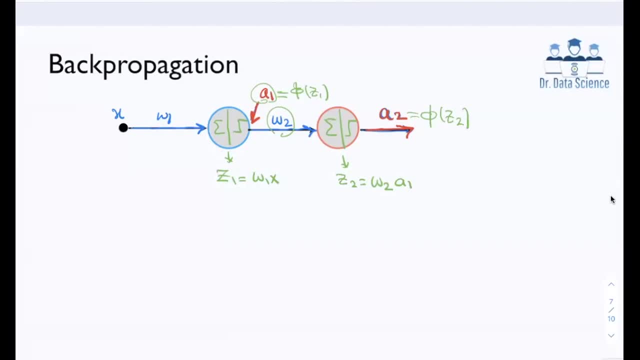 And A1 is phi of Z1.. So I tried to make this as simple as possible. We have two weights, W1 and W2, and then we have these outputs, A1 and A2.. And the rest is basically using. we have using these simple linear equations. 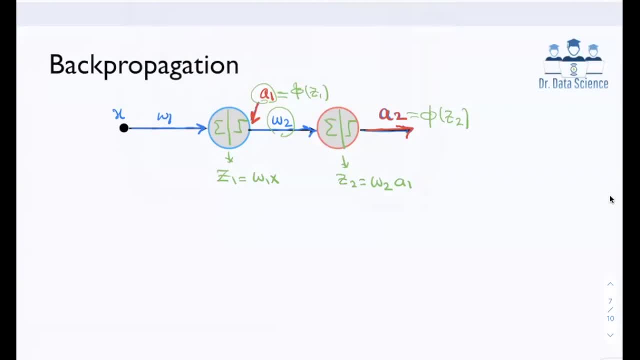 So the other thing that happens because most neural network models are using supervised learning. So this A2, is what the neural network produces, And we have also a target value, which is Y. So this is the actual output value that we like to see. 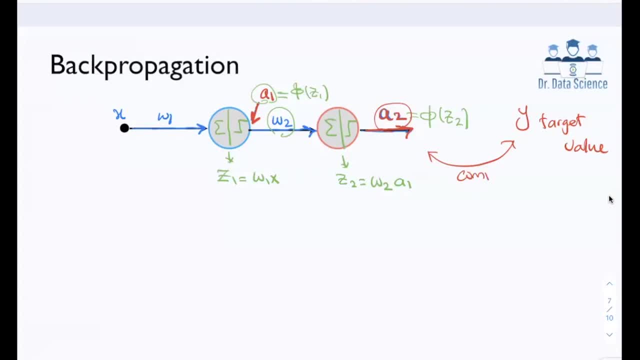 And we usually compare these two things compare using some cost function. let's call it C Then in this case I assume a simple function. We just use sort of like a mean square type. error: We just subtract A2 by Y. 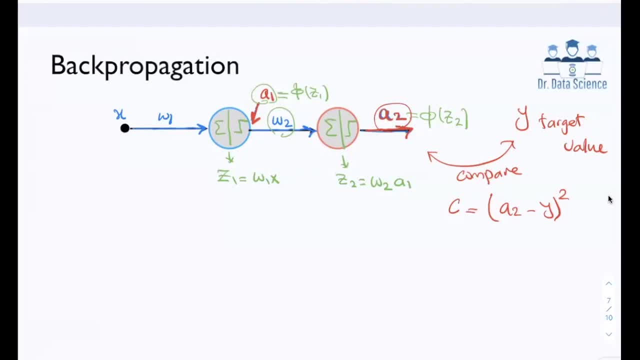 and we take this to the power of Z. So that's exactly what happens in the mean square error for regression problems. So now, in order to update these weights, like W1 and W2, we need to use partial derivatives because obviously we have more than one variable. 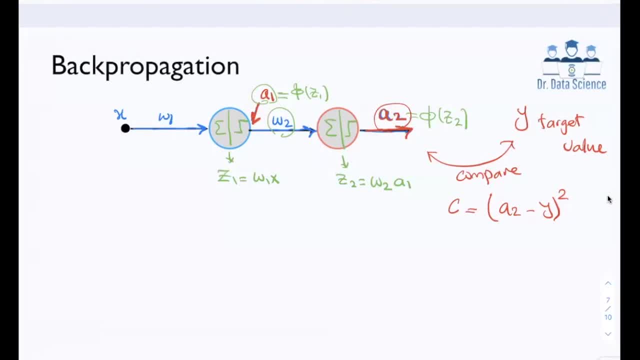 And also we need to be able to find these partial derivatives of the cost function with respect to these weights. So the first thing that we want to do here is to find the partial derivative of C with respect to W2, right, This weight that goes to the output layer. 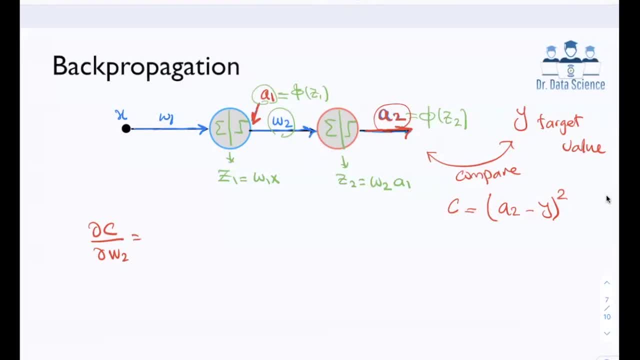 So obviously that's a complicated problem. So, in order to simplify this, we use something called chain rule, And it is very easy to use. In the way that you can think about it is that I always like to create this, what is called computation. 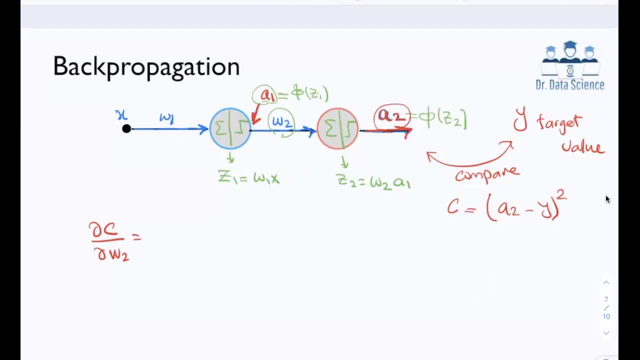 This is a computation graph, right? So we have this A2 and we have Y, and these two they give us C, because C is equals to A2 minus Y, to the power of two, And A2 is given by Z2, and Z2 is given by W2 and A1.. 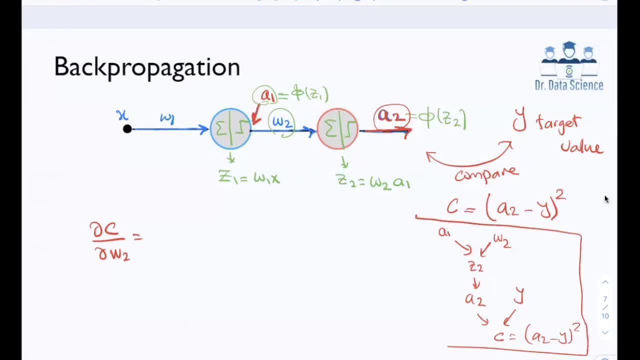 So just have this in mind. So now, if I want to find the partial derivative of C with respect to W2,, I can find the partial derivative of C with respect to A2.. Partial derivative of A2 with respect to Z2 and Z2 with respect to W2.. 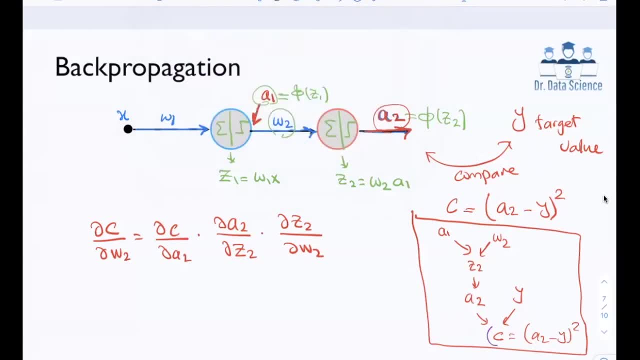 So this is the path that we took here, right? So we started from here, then we went here right, Right then here, and then we went here, So we find all these partial derivatives. So now let's look at this. 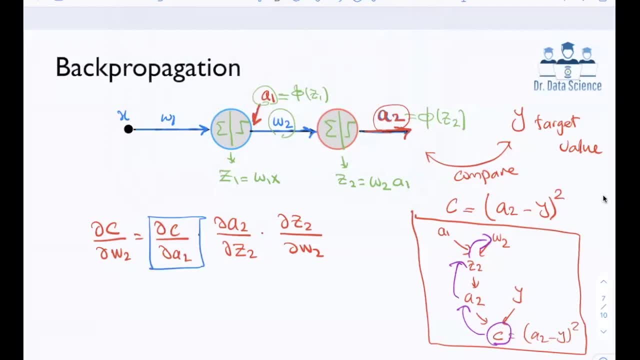 So what's the partial derivative of C with respect to A2?? So this is a quadratic again term, right? So what you can do is that you can call these, let's say anything you want. I call these like B. What's the partial, what's the derivative of B squared? 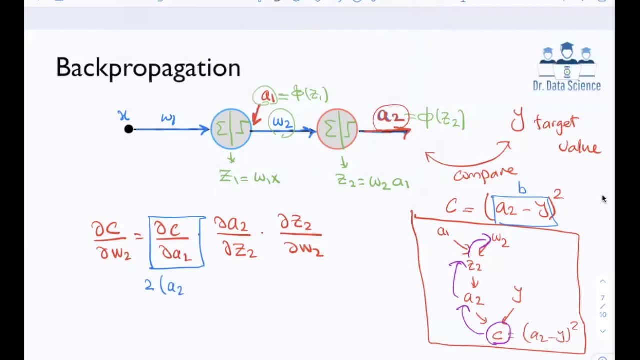 A2 times B, and remember B is equals to A2 minus Y. And now you have to take the derivative of the inside these parentheses, B with respect to A2, which is one, because derivative of X with respect to X is one. And then now the second part here is: what's the derivative? 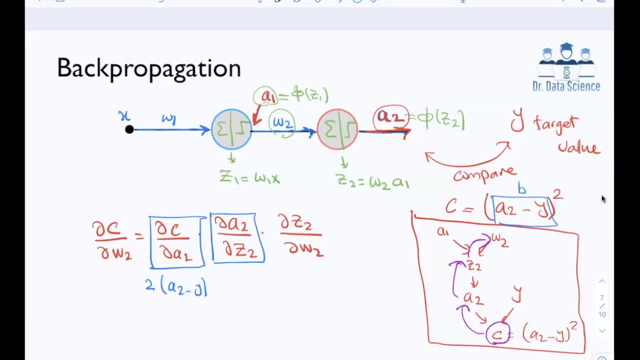 of A2 with respect to Z2?. So now we can use this equation here for that. So that's just simply the derivative of this function, phi, calculated at the point Z2.. And then, for the last one, we use this equation that we have here: 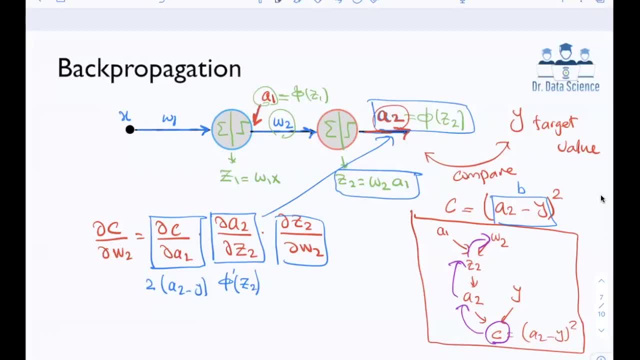 that the partial derivative of Z2 with respect to W2 is equals to A1. So why did this happen? So, again, that's the part that we have this partial derivative that you have to consider. So I want to find the partial derivative of this term. 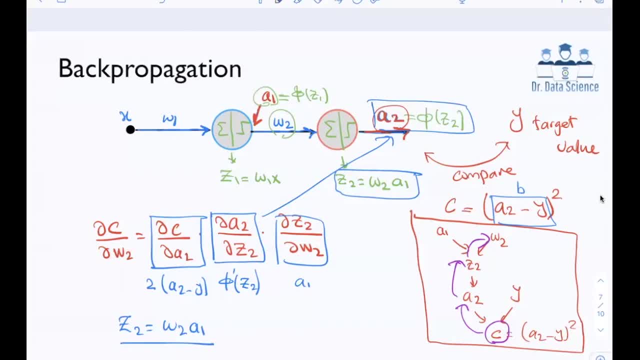 with respect to A1.. So I want to find the partial derivative of this term with respect to A1.. Sorry, with respect to W2, that was the problem, right. So you want to find the partial derivative with respect to W2.. 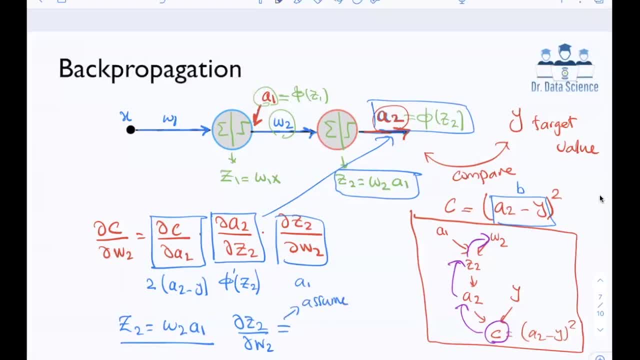 So we assume A1,, which is the other variable, is constant Right, And we know that if I have like two times X, what's the derivative with respect to X? Is two right Is the constant that is next to X. 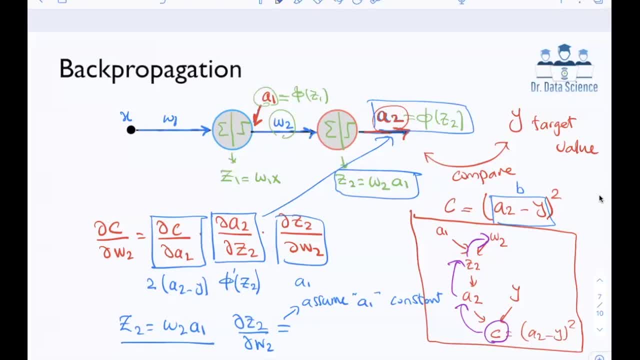 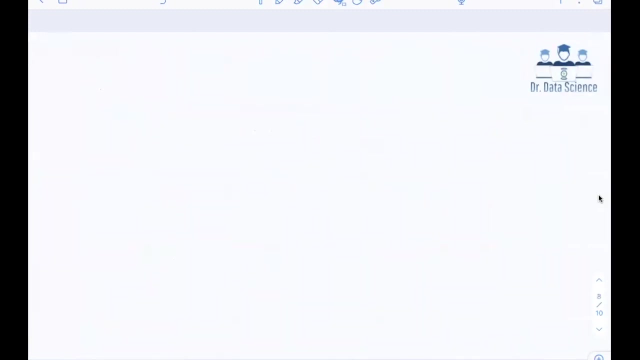 So here, if I want to find the partial derivative of Z2 with respect to W2, we need to pick this constant that is next to it, which is A1.. So I can just copy this now and go to the next slide, right? 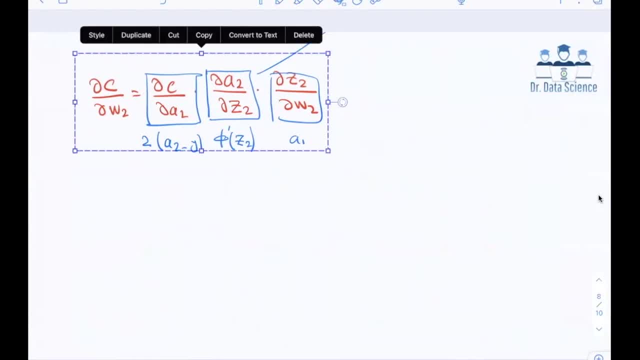 And go to the next slide right. So that's like what I found previously, that the partial derivative of C with respect to W2 is equal to A1.. So that's like what I found previously, that the partial derivative of C with respect to W2 is equal to A1. 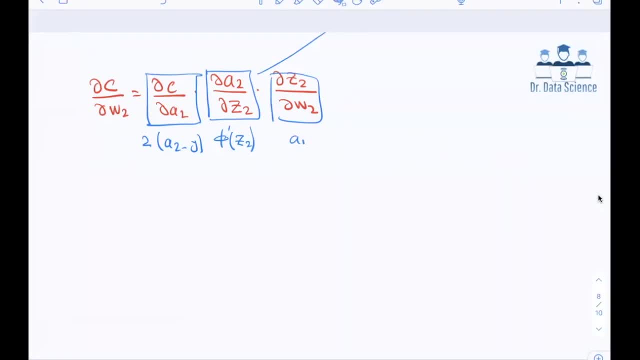 So that's like what I found previously, that the partial derivative of C with respect to A1 equals to multiplication of these three terms, And let me also again draw that computation graph that we have. So that's a good practice. So, if you remember, we said that we have A2,. 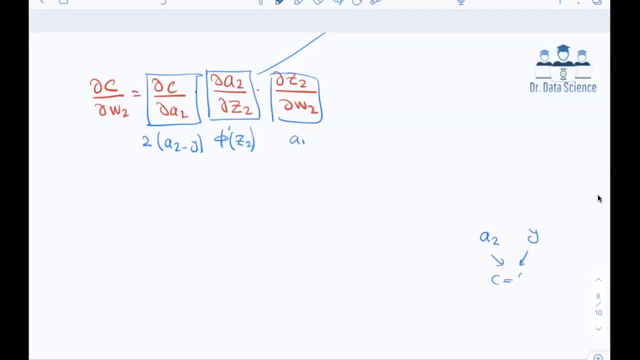 we have Y right, So we had the cost function, which was A2 minus Y to the power of two. A2 is related to Z2.. And Z2, if you remember, is connected to W2 and A1.. It's related to W1 and Z2, so we need a 20 percent effect. 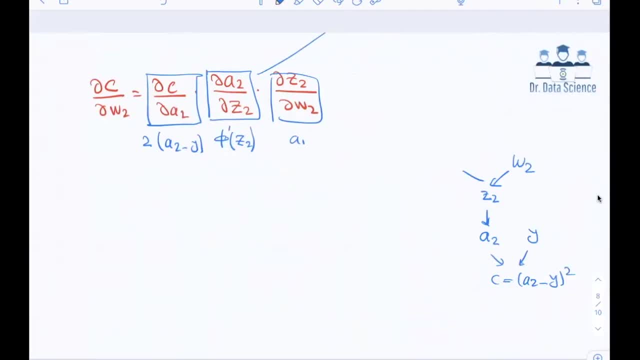 a1 right. so now let's look at partial derivative of C with respect to a1. so in this case I get partial derivative of C with respect to a2. I go step by step: a2 with respect to z2 and z2 with respect to a1- and here's where the magic. 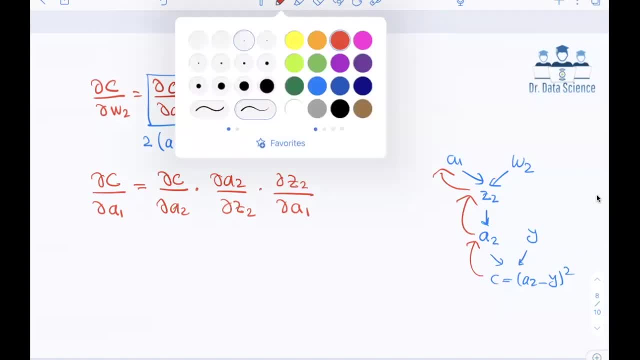 happens. if you look at it, we already calculated two out of three terms that we have here, so this means that now I don't have to just start from scratch. I can just use these results that I have for both cases, and the only thing that is extra here that I have to calculate is this term right and 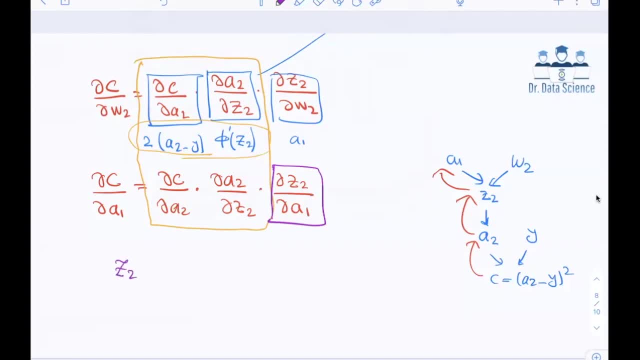 let's remember what was z2. if you remember from the previous slide, z2 is equals to w2, a1, and now we have to again use the partial derivative. so we want to find the partial derivative of C with respect to a1, and we have to again use the partial derivative, so we want to find the partial derivative of. 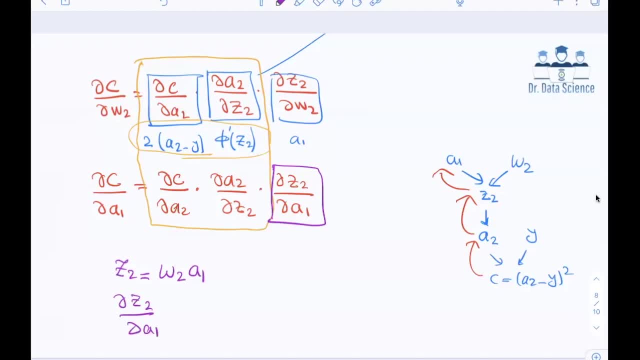 z2 with respect to a1. so this means that we assume w2 is constant and when we have a constant times a variable, the derivative is that constant. so this means that this partial derivative is w2. so now we have the partial derivative with respect to a1 and we can continue this process. 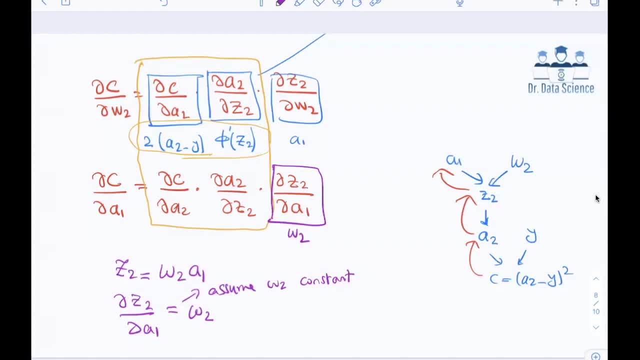 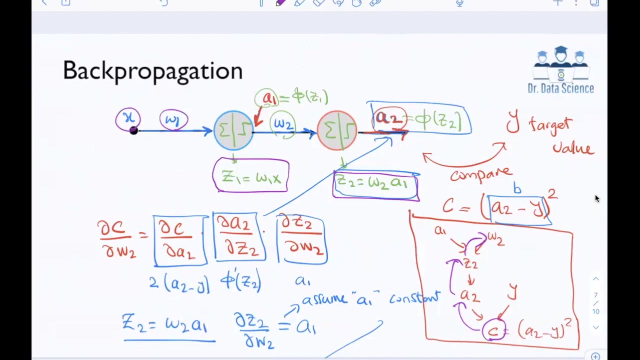 to find all these partial derivatives? How So, if you look at that, a1 is connected to z1 and z1 is connected to w1 and x, right? So let's look at it to make sure that we did this correctly. So, if you look at that, z1 is equals to w1, x, where w1 is the weight, x is the input. So that's what.